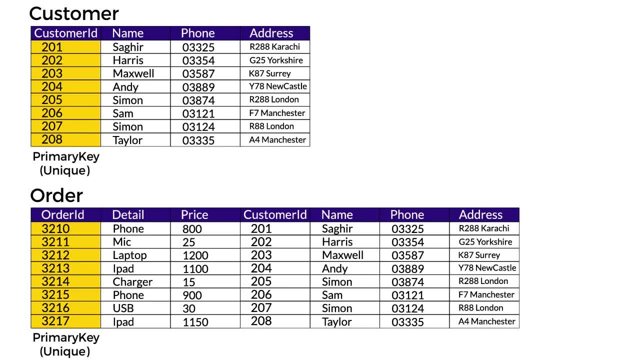 a big no-no in database. Other thing is that it's data redundancy. There is already a customer table and that contains all properties. So data redundancy slows down the process of database, which is again a big no-no for database. So what we can do in a one-to-many relationship and linking them, we will make absolutely. 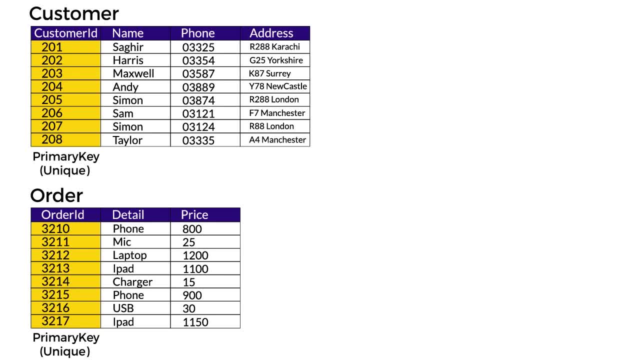 no change in the one side of one-to-many relation, which is customer, and we'll add a column to the other side of the table, which is order. here taking primary key of the customer table and adding it to the order table, which will act as a foreign key. Now, foreign key just. 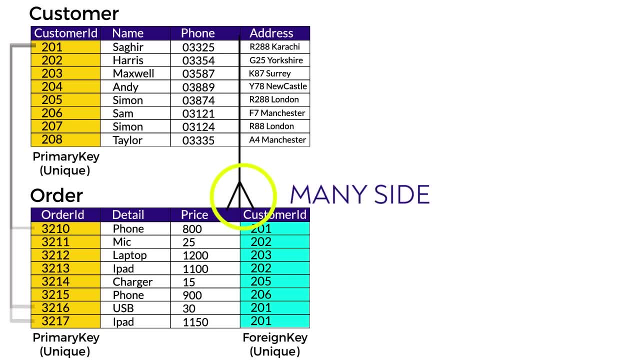 to remind you, primary key numbers cannot be repeated, but foreign key numbers can be repeated. That's how we'll create the link between one-to-many table. Now the tables are linked by the virtue of foreign key. Foreign key is the primary key of the customer table. 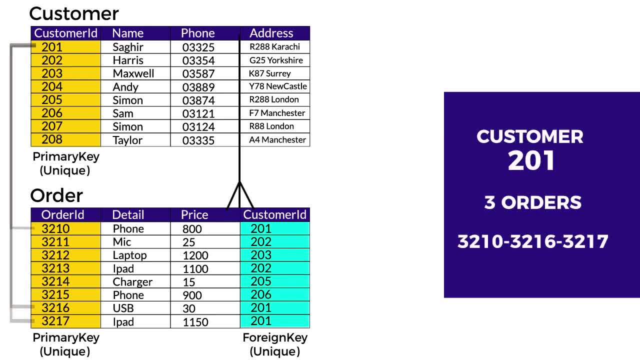 We can see from this table, if we need to know how many order table is there, We are going were made by 201 customer. we can see from the order table it's 3 2 1 0. 3 2 1 6. 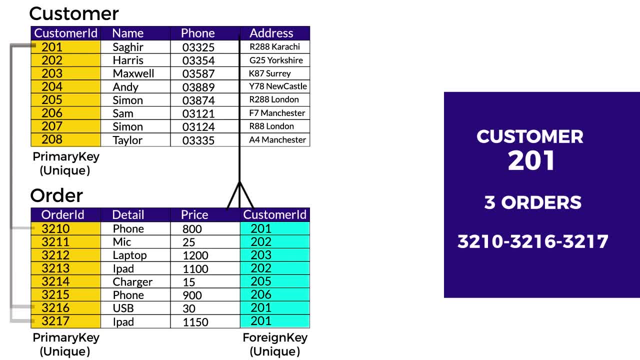 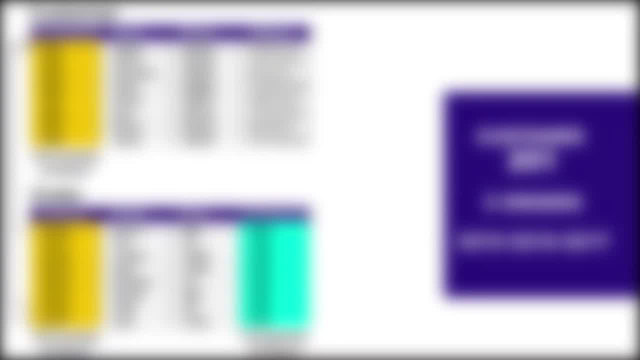 and 3, 2, 1, 7, 3 orders were made by customer 201 and vice-versa. we can find the details of the owner of the order in this table. customer is the one side and order is the many side. one customer can can have many orders but one order. 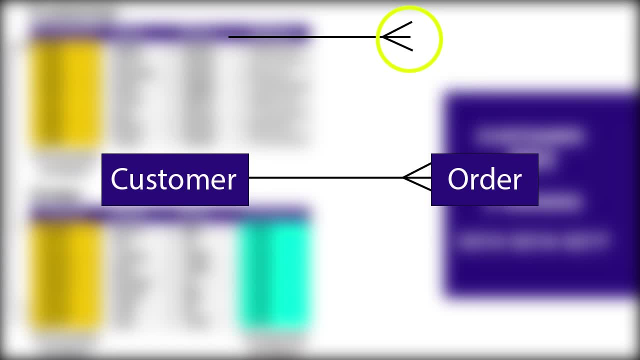 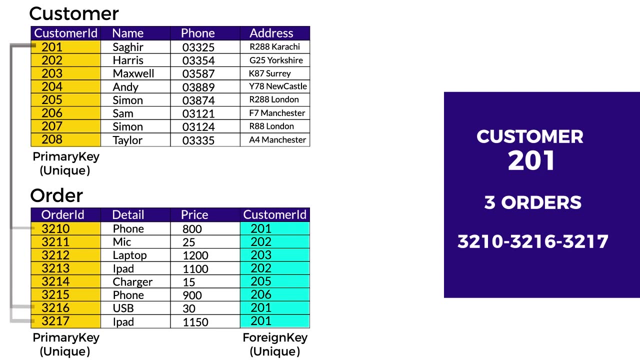 cannot be made by many customers, like order number 3, 2, 1, 0 cannot be made by many customers. it can only be made by one customer. another example: customer 202 has two orders. with the help of two tables we can find the order details of. 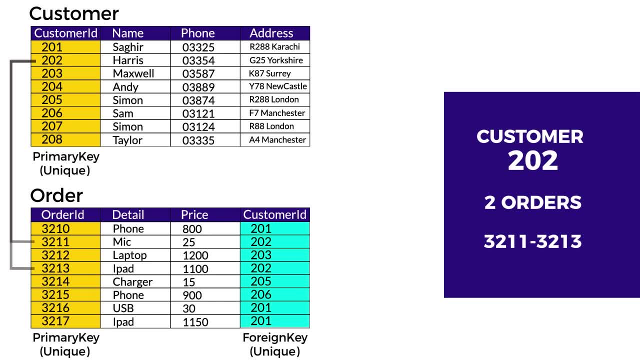 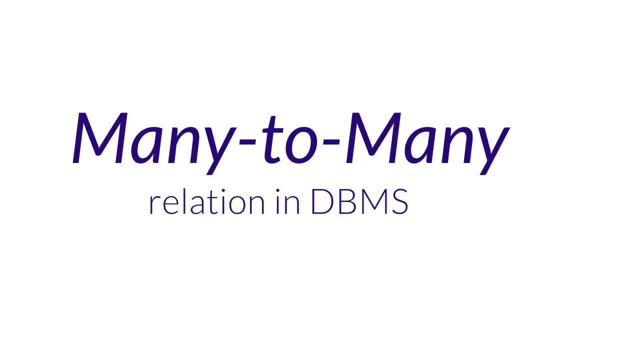 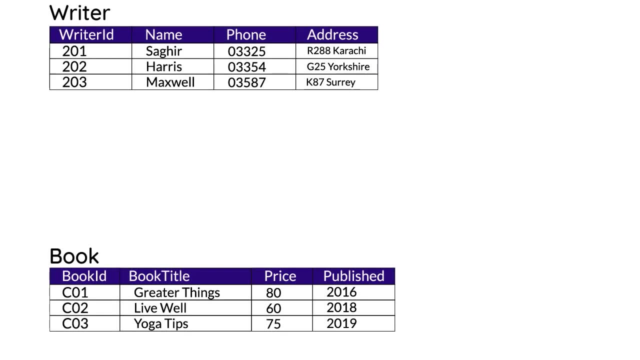 any customer or customer details of any order in this case, and both tables are linked by foreign key many-to-many relationship. we'll use the example of writer and a book. a writer can write many books and one book can be written by many writers. on both end side there's 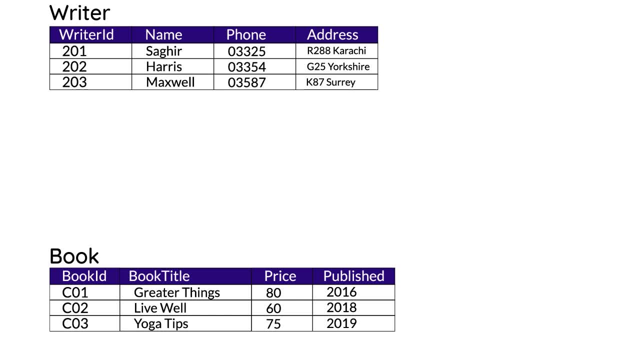 a many-to-many situation example. we have a table of a writer and a book writer has a primary key of a writer ID book as a primary key of book ID. it cannot be linked with the foreign key because it will only consider one side as many and